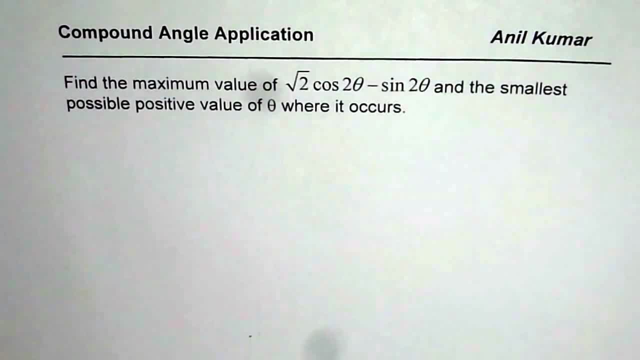 I'm Anil Kumar and here is a very interesting application question where we are going to use compound angle formula. The question here is: find the maximum value of square root 2 cos of 2 theta minus sin 2 theta and the smallest possible positive value of theta where it occurs. 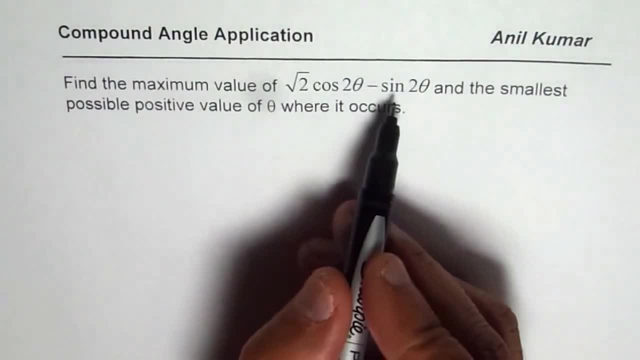 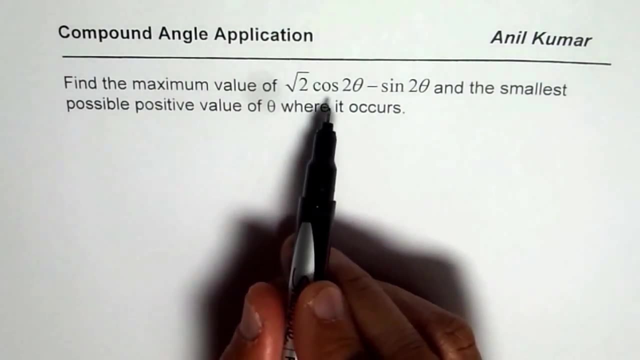 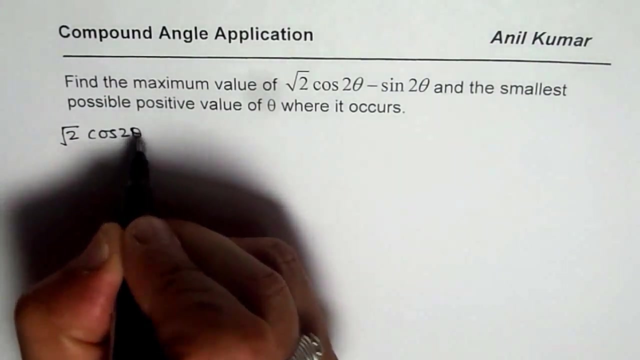 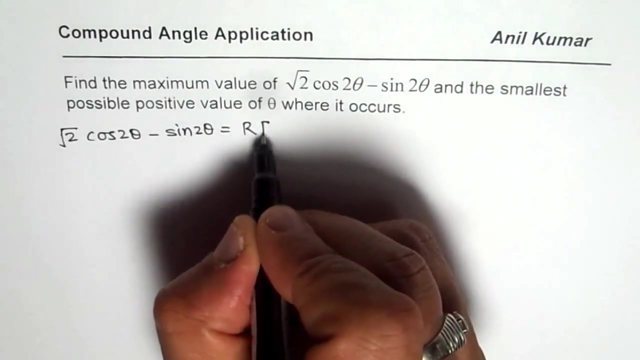 Now to find maximum value of this, first step should be that we should be in a position to write this as one trigonometric function, and that is what we will learn in this video. So we have square root of 2 cos of 2 theta minus sin 2 theta. We could write this as r times cos of 2 theta minus alpha. 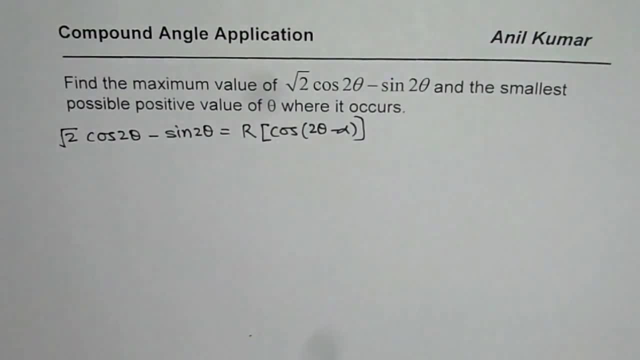 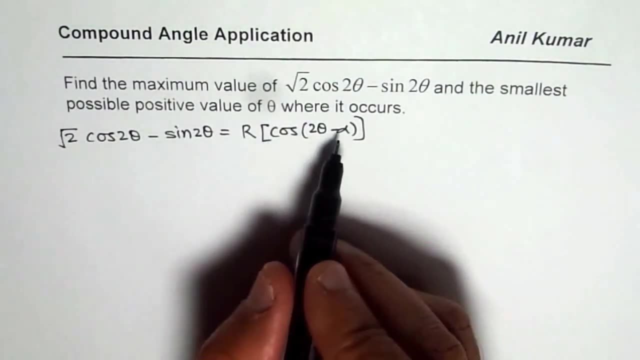 We will write it as r times cos of 2 theta minus alpha. We will write it as r times cos of 2 theta minus alpha. We will write it in one trigonometric ratio, cos, And then we will find the maximum. This is a very good technique, and let us see how to apply this technique. 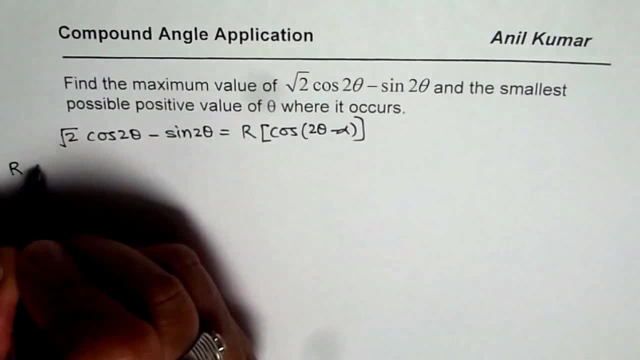 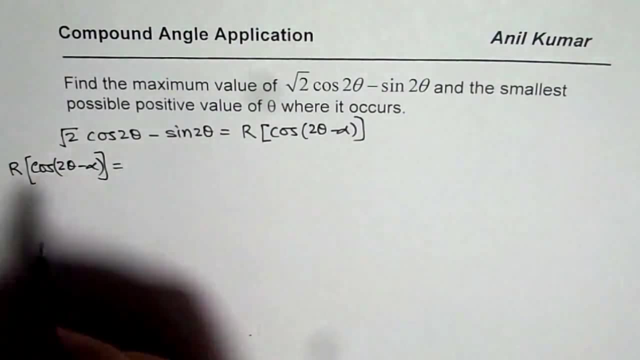 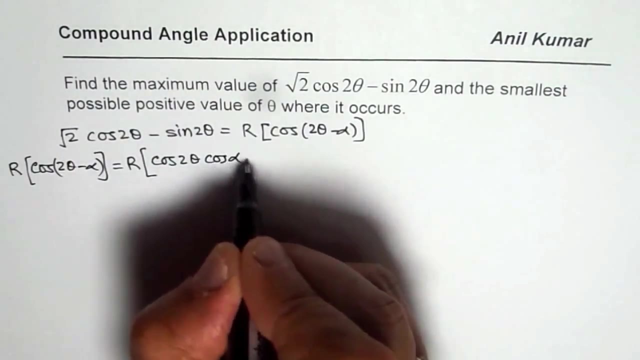 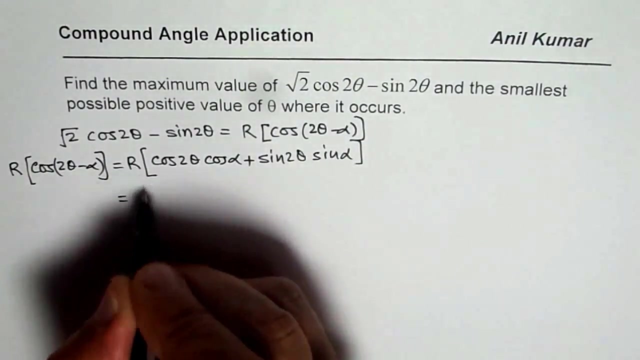 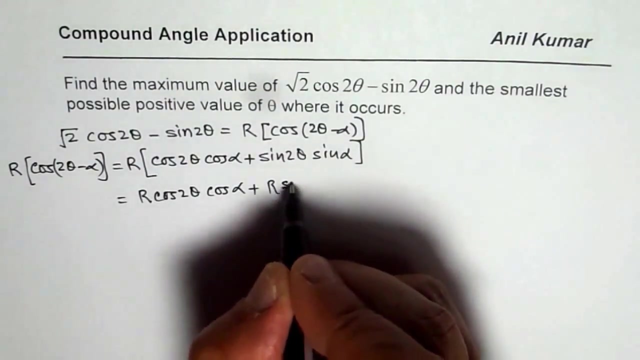 Now let us begin with r of cos 2 theta minus alpha. Using compound angle we can expand this, so we get r times cos 2 theta, cos alpha, plus sin 2 theta minus sin 2 theta. So when we expand it we get r cos 2 theta, cos alpha, plus r sin 2 theta, sin alpha. 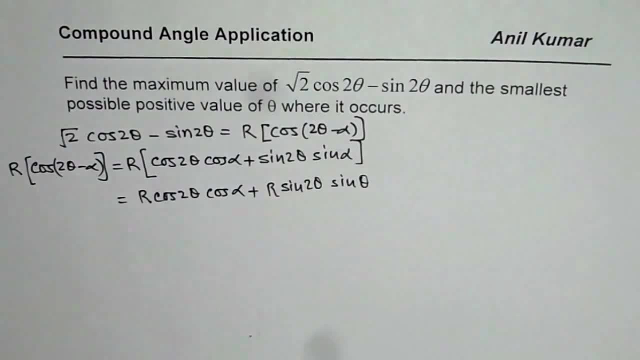 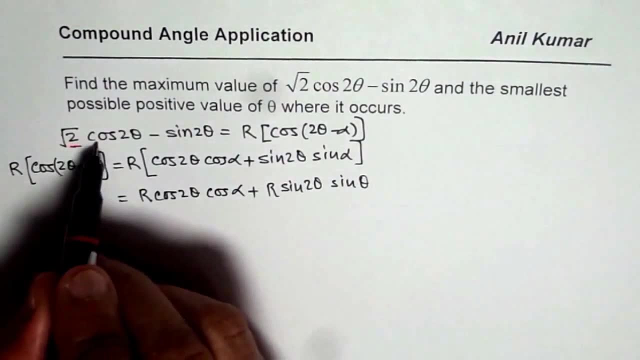 Now, if you compare this equation with what we have here, you will find that cos 2 theta, cos 2 theta is there. So what we can write here is that r cos 2 theta, cos 2 theta is there. So what we can write here is that r cos 2 theta, cos 2 theta is there. 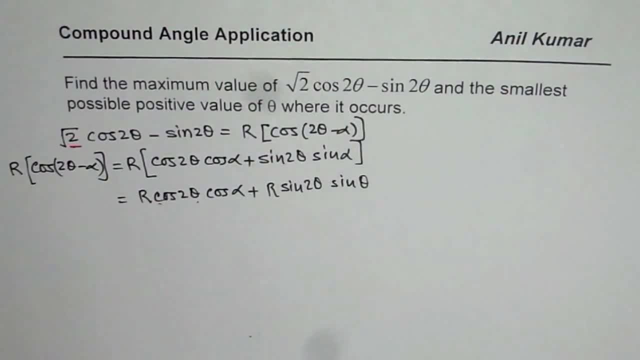 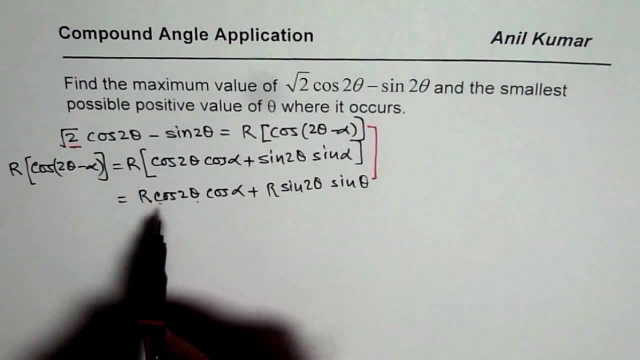 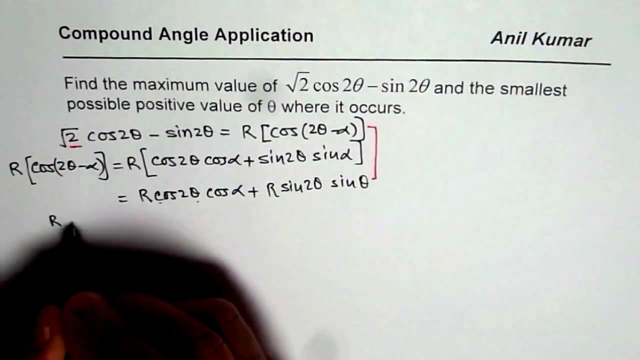 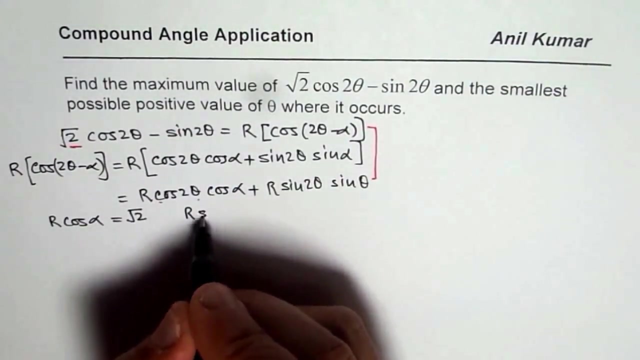 what we can write from these two comparisons. So now let us compare these two parts. I mean square root, 2 cos 2 theta with r cos 2 theta cos alpha. In that case we can write r cos alpha as equals to square root of 2 and r sin alpha. this is alpha, sin alpha as equals. 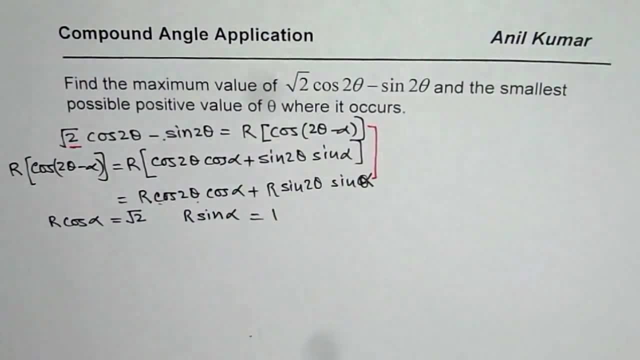 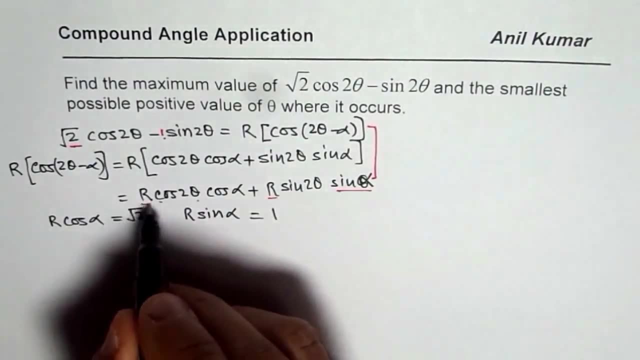 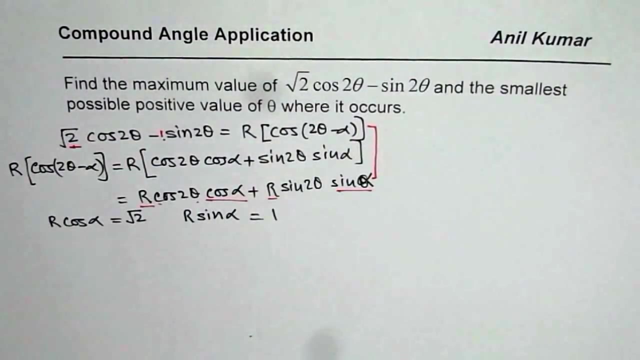 to 1.. 1 is the coefficient there. Do you get the idea? So if you compare, we can write r sin alpha as 1 and r cos alpha as square root of 2.. We already have cos 2 theta and sin 2 theta. So when we compare left side and right side, we could write our equation like: 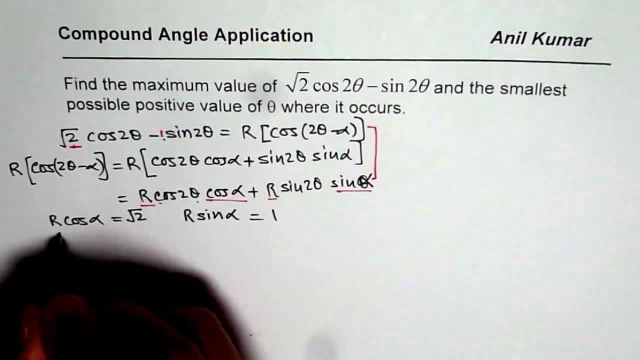 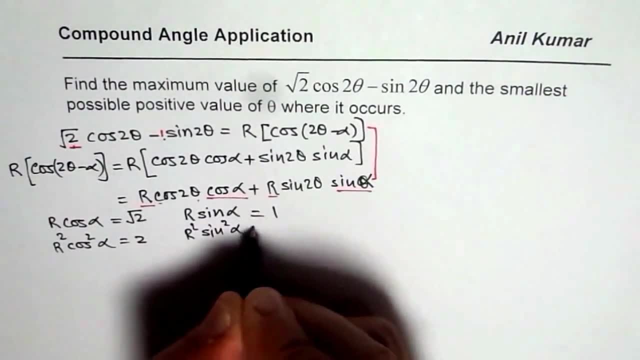 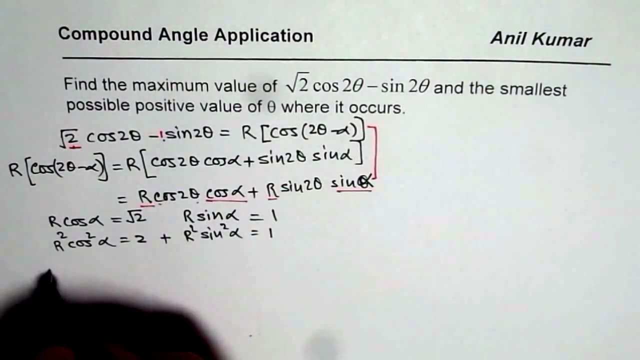 this. Now let us square both of them. If we square, we get r square cos square root of 2, and r square sin square alpha equals to 1.. And if I add them up? if I add them up, then what happens? 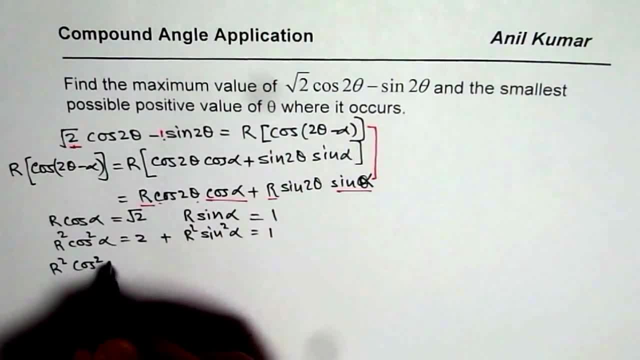 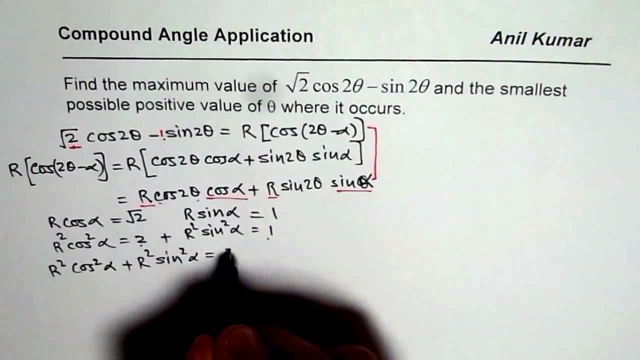 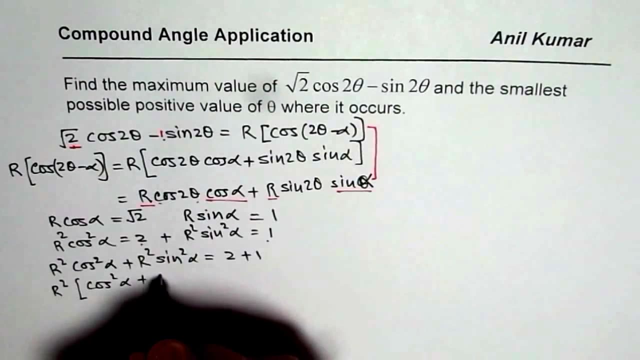 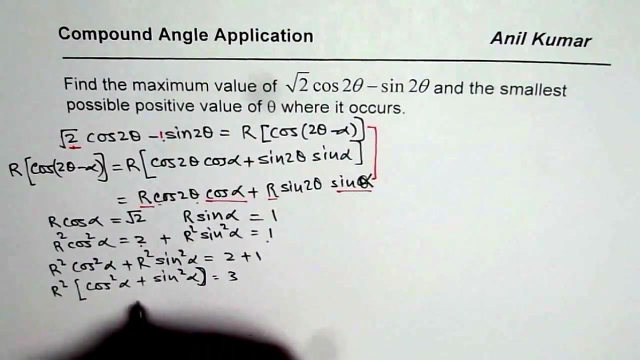 We get r square cos square alpha plus r square sin square alpha equals to 2 plus 1.. Taking r square common, we can write this as: cos square alpha plus sin square alpha equals to 3.. So r r cos square alpha plus sin square alpha is 1. So therefore r square is equals. 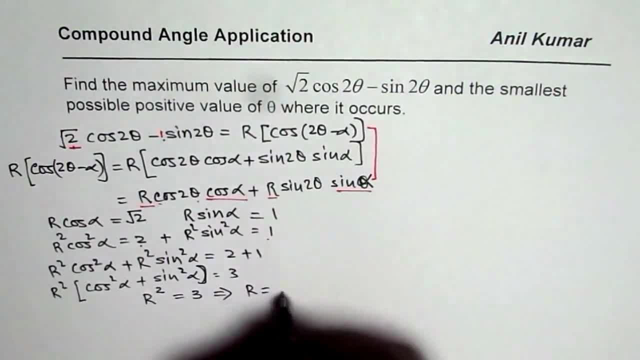 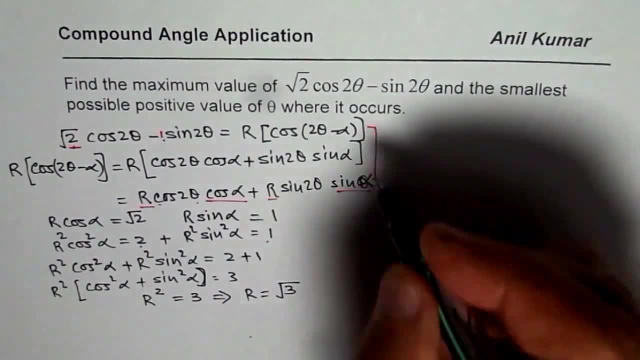 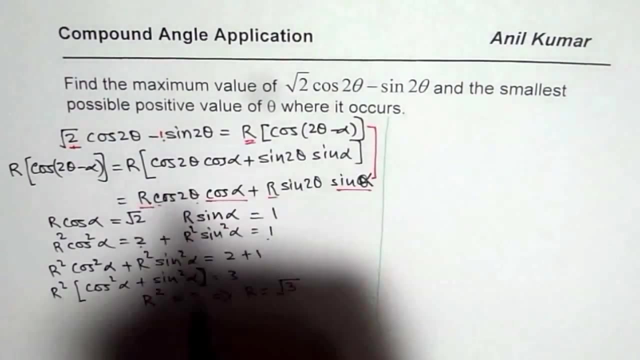 to 3, and that gives us r as equals to square root of 3.. Now, whenever we write this equation, we take r as positive number, So that is how we get the value of r. So let me write down clearly what is r for us in this equation. So we found r as equals. 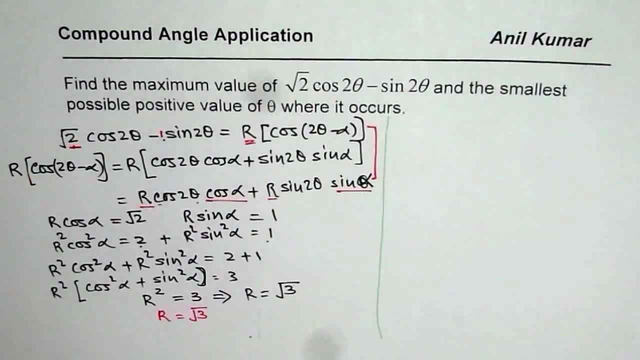 to square root of 3.. Now to find alpha. what we can do is we can divide one equation by the other. So to find alpha, what we are doing here now is we are taking help of these two equations and we will divide r for sin alpha by r cos alpha, So r sin alpha is equal to 1.. Now here, 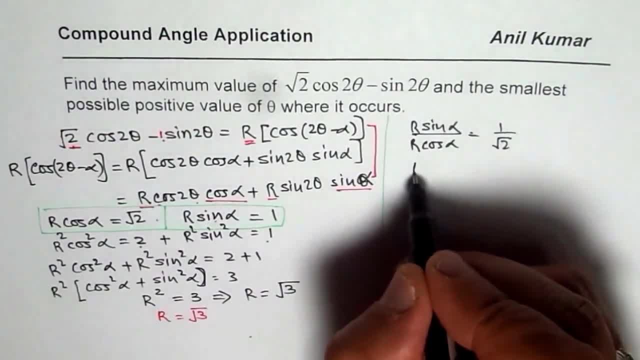 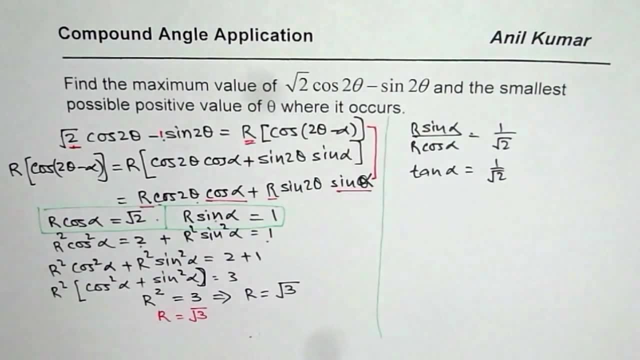 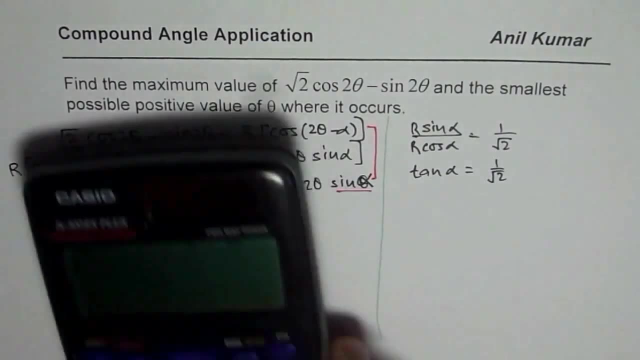 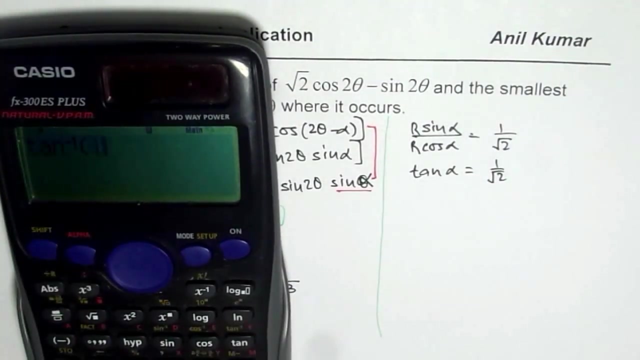 divided by square root 2.. So we get tan alpha as equals to 1 over square root 2, and the acute angle for alpha which will give us 1 over square root 2 is- let's use the calculator right. So what we have is tan inverse of 1 over 1 divided by square root 2, bracket closed equals to. So we get. 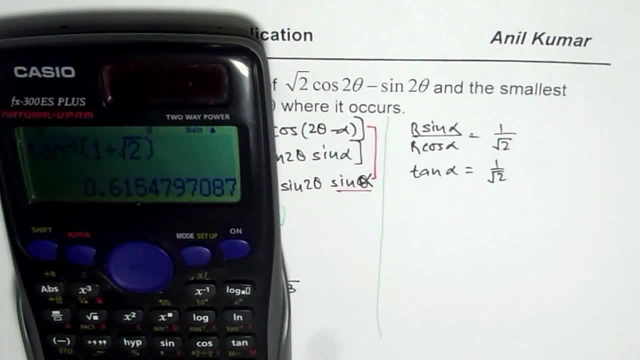 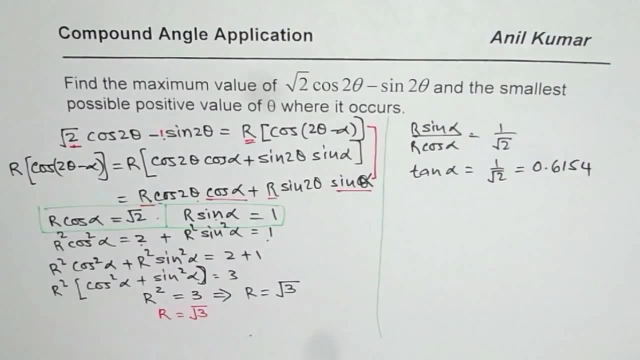 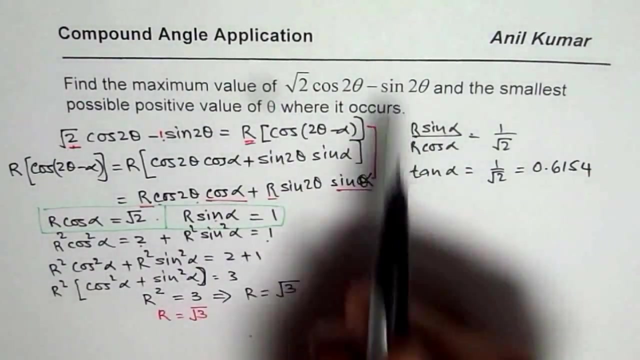 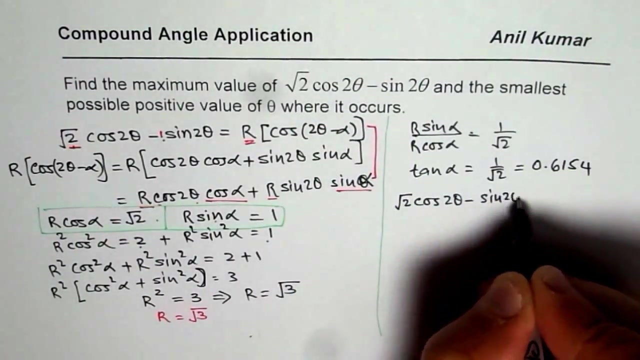 0.6154.. So we get this as equals to 0.6154, right? So that is the value of alpha for us, and therefore we can write now the expression which was square root of 2 cos, 2 theta minus sine 2 theta, as: 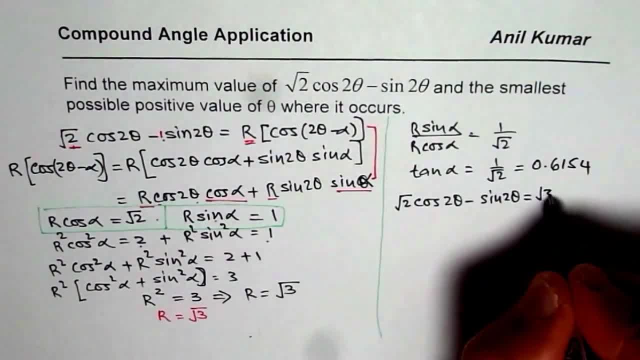 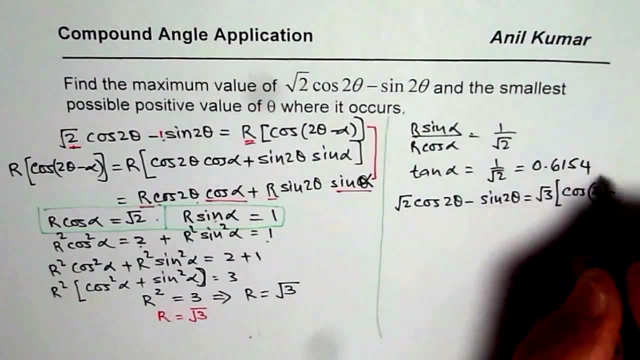 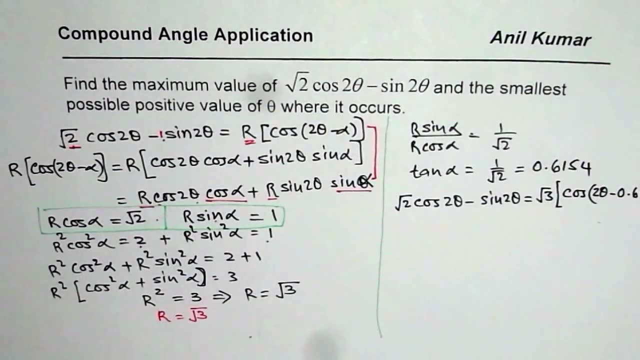 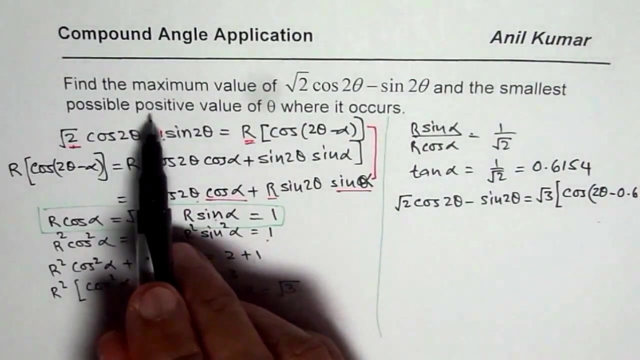 equals to r squared root, 3 square root of 3, cos of 2 theta minus 0.6154. right, So that becomes our expression in single trigonometric ratio. Now, now we need to find the smallest possible positive value. We need to find the maximum value of this. 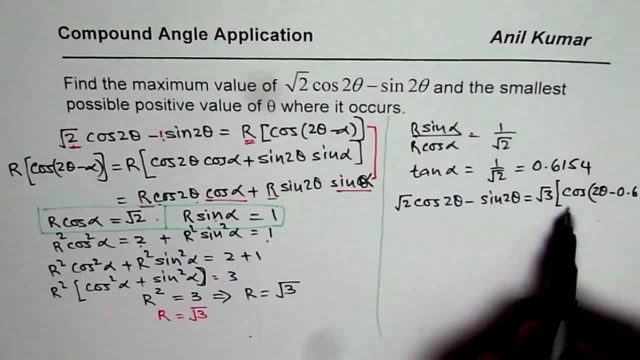 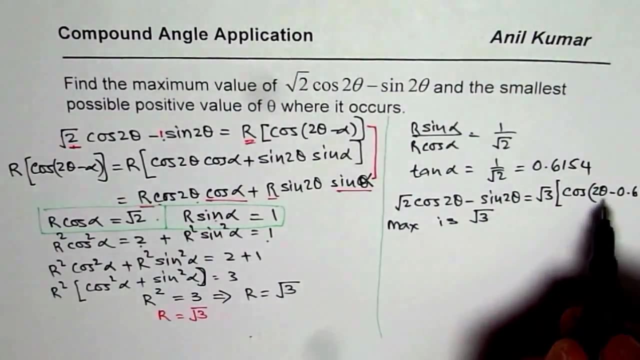 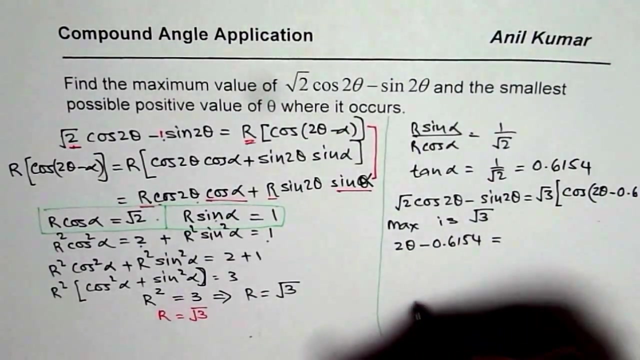 function. Now the maximum value can occur, which I mean cosine function can have maximum of 1 only, right. So we know from here that the maximum is square root of 3, right. And that will have occurred when 2 theta minus 0.6154 is equal to 0, right. Only then the maximum is going to. 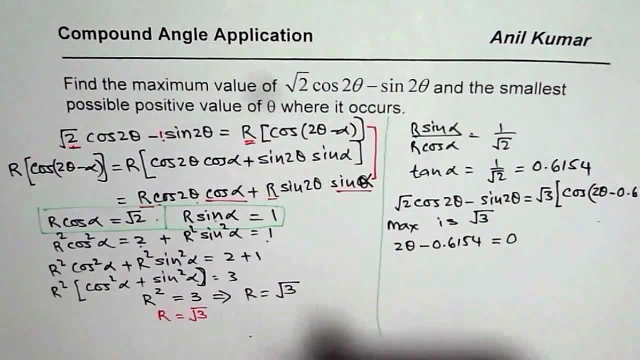 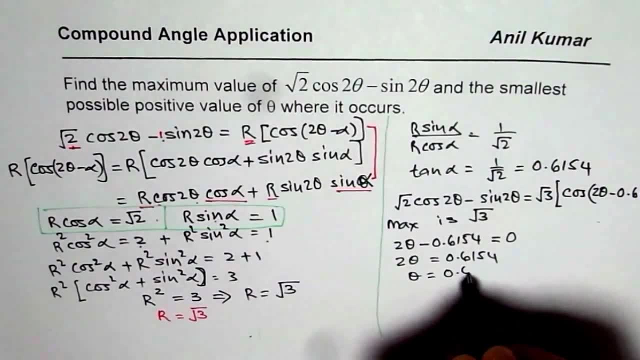 occur right. So from here we can find the value of theta. So we get 2 theta equals to 0.6154, or theta equals to 0.6154 divided by 2.. So let's divide this by 2.. 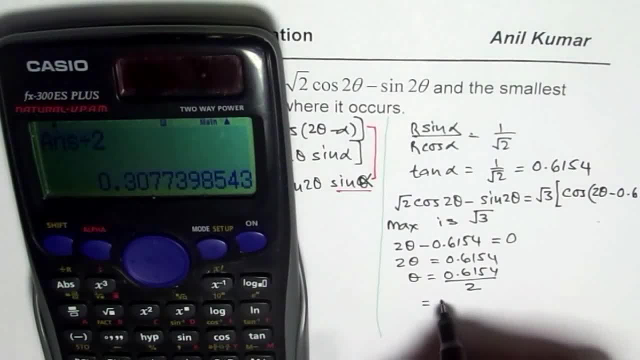 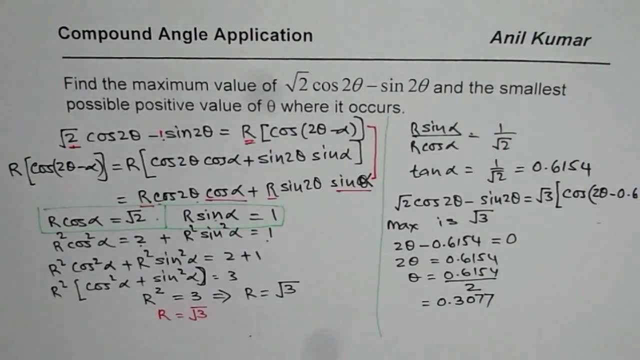 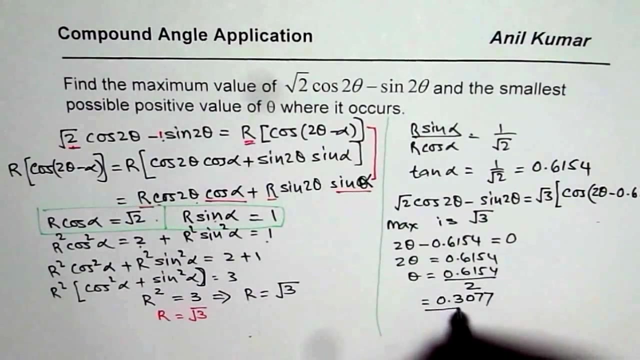 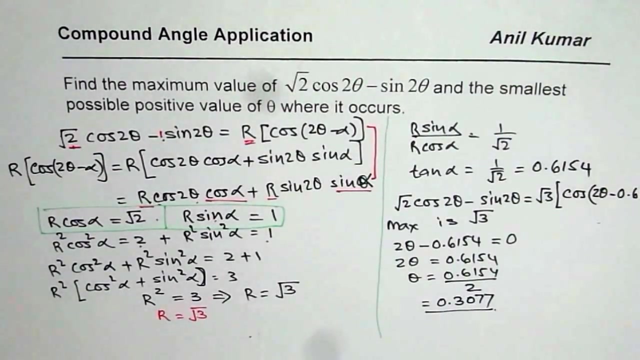 So we get theta as equals to 0.3077,. right, So that is the value of theta for which this particular function will have the maximum value. right, So that is our answer. right, So that is how we can actually solve such questions. I hope that helps. So the strategy here is to write down: 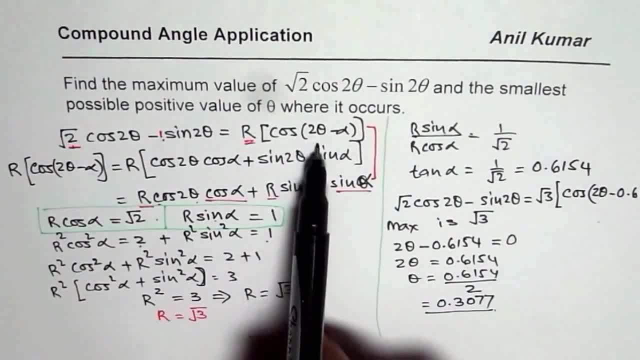 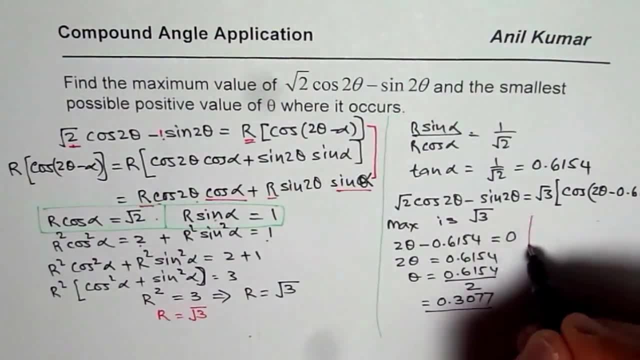 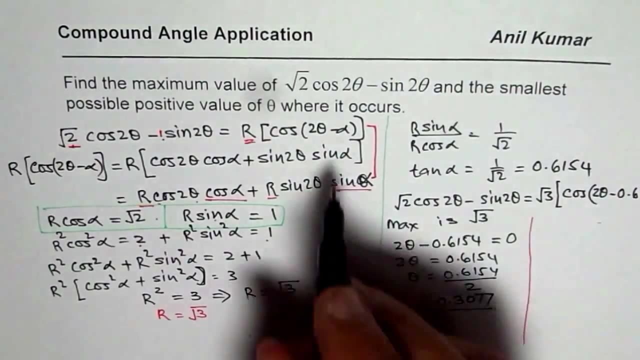 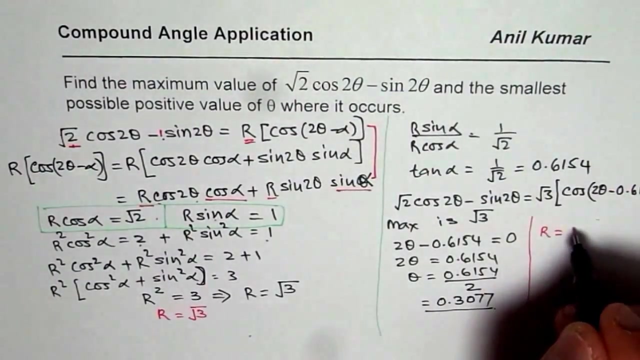 these functions as a single cosine function and then find the maximum. And key which we find here is that we could write all these functions as r cosine theta or 2 theta, whatever this argument is minus alpha, where r is equals to these coefficients right a square. let's say the coefficients are a and b.